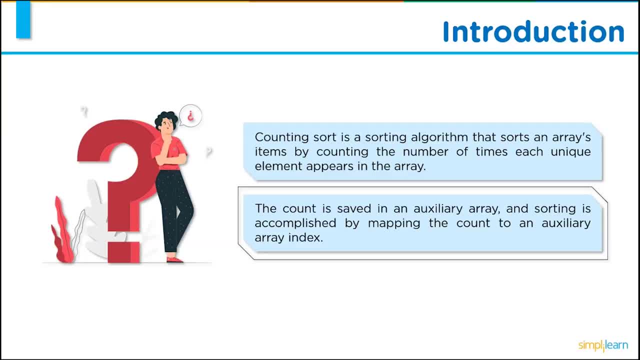 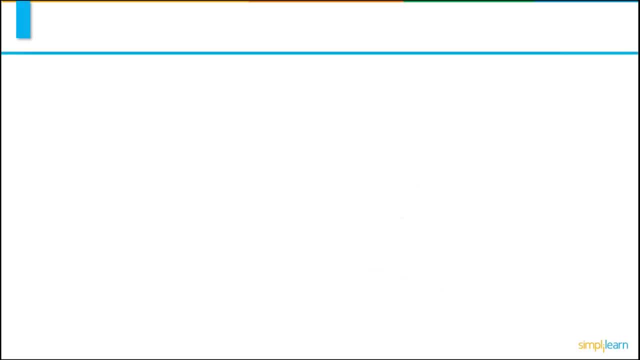 and the sorting is done by mapping the count as an index of that auxiliary array. Now let's discuss the counting sort algorithm. Let's say we have an array. First we will find the largest element in this array to evaluate the range of the elements. 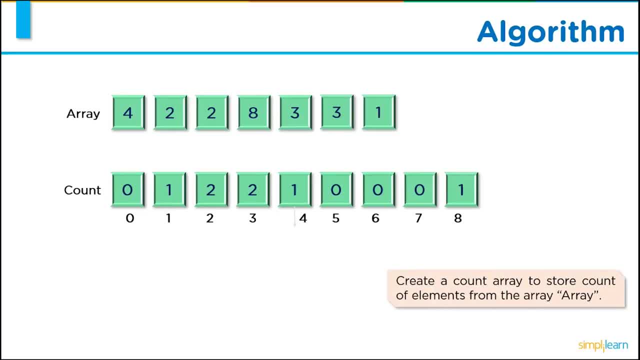 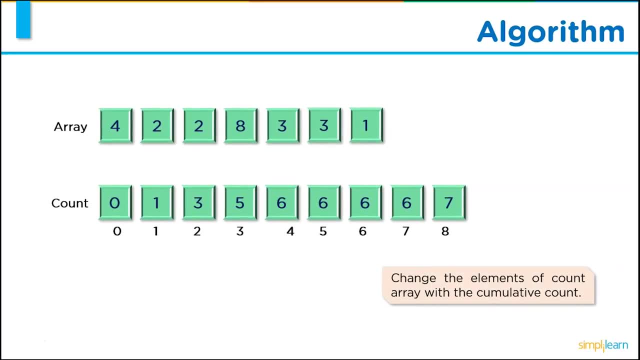 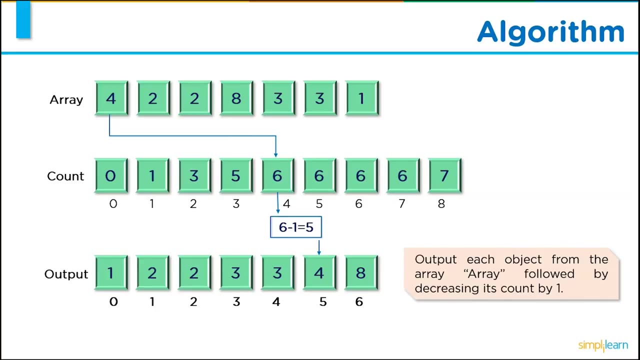 Then we will create a count array to store the count of element from the array. Then we will update the count array's element with a cumulative count. At last we will output each element from the array, followed by decreasing its count by one. 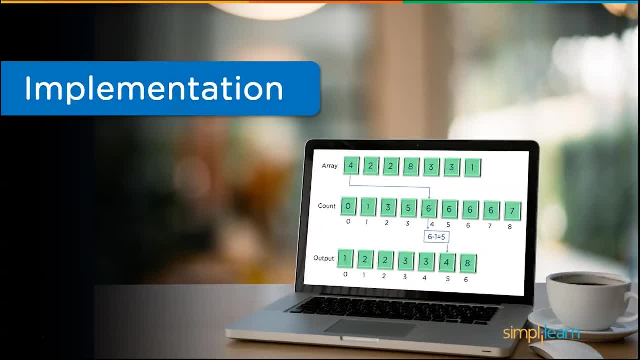 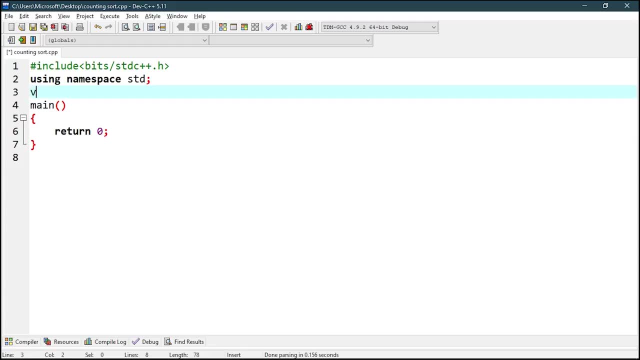 We have now introduced the counting sort and its algorithm. Now let's try to implement this algorithm in the code editor. Let's start by creating a count sort function. void count sort. It's argument as int arr, int n, We will declare an array output. 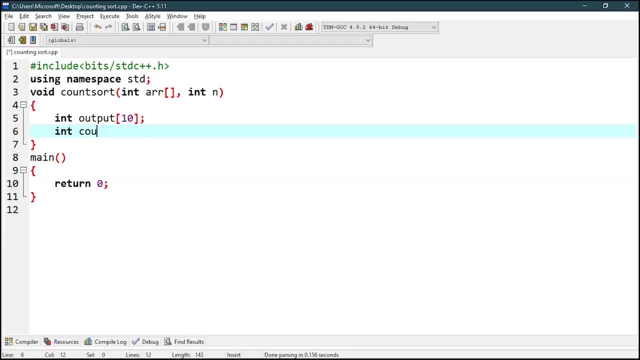 with size 10 and an array count again with the size 10.. And an integer variable, max, is equals to arr at zero. Now we will write a for loop to find the largest element of this array. So for int i is equals to one, i less than n, i plus plus. 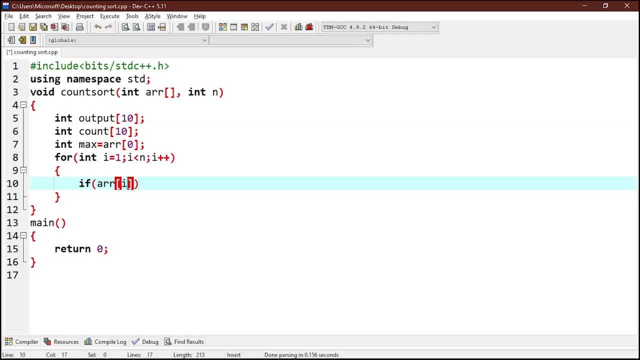 If ARR at i is greater than max, then max will be equals to ARR at i. Now we will initialize the count array with all zeros. So for int i is equals to zero to i less than equals to max. plus plus i count at i is equals. 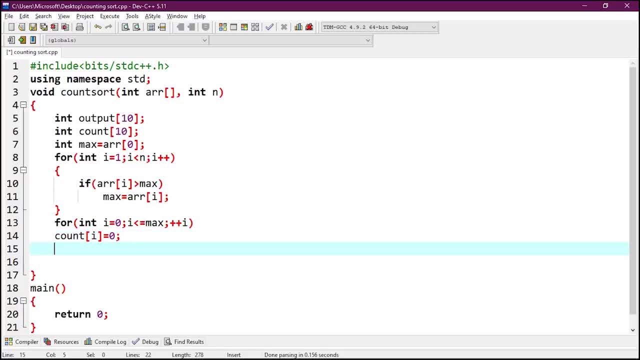 to zero. Now we will store the count of each element in this array. So for loop: int i is equals to zero. i less than n. i plus plus count at ARR bracket: i is plus plus. Now we will write a for loop to store the cumulative count of each array. 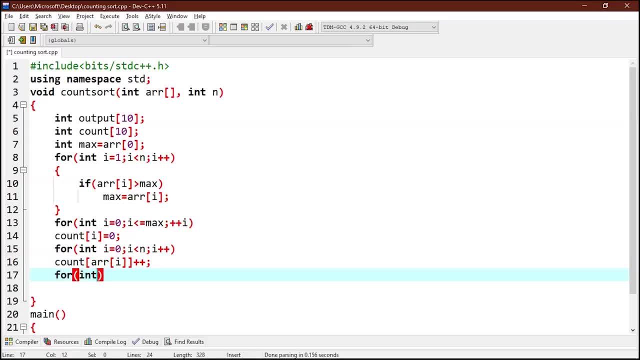 So for int i×1, Where i is less than equals to max at i++, count at i is equals to plus. where i is less than equals to max at i++, count at i is equals to plus. equals to count at i minus one. now we will find the index of each element of the original array in count. 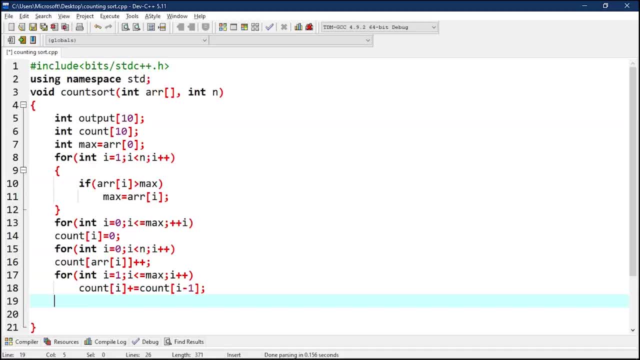 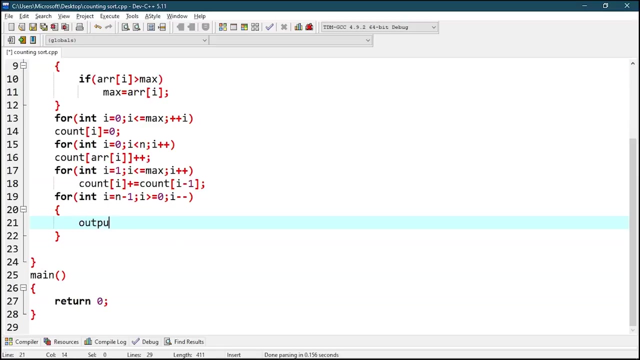 array and place the elements in the output array. so for int i is equals to n minus one. i greater than equals to zero i minus minus. so output account at ARR i minus one is equals to ARR at i, and then we will decrease, count ARR i by one. 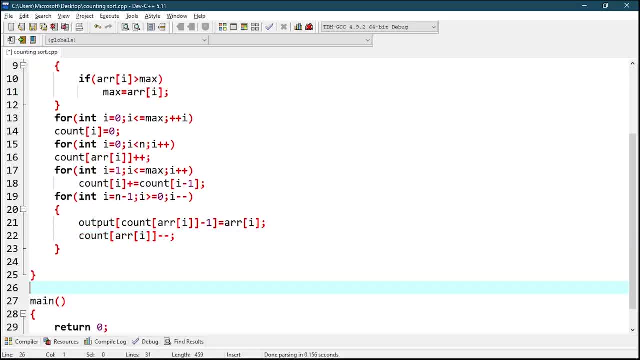 now let's write a function to print this array, so void: print array. so int ARR, bracket comma: int n. so for loop, int i is equals to zero. i less than n. i++. cout ARR at i and then we will decrease. count ARR at i. i less than n. 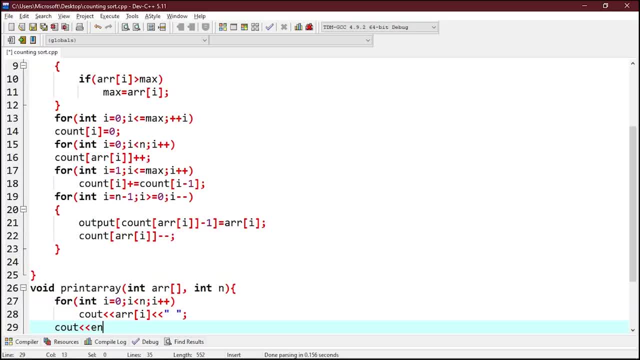 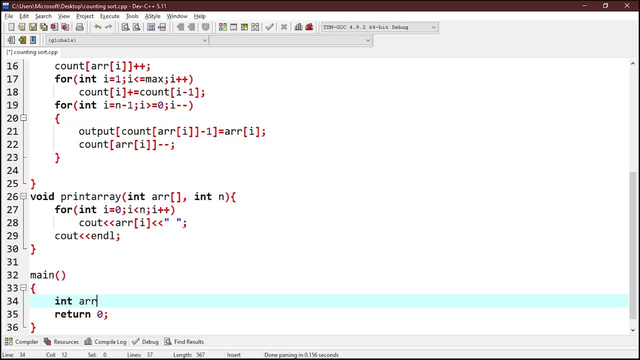 out. and now let's write the main block. int arr is equals to- we will write the element. now let's find out the size of this array. so int n is equals to size of array divided by size of array's first element. now we will call the count sort function. 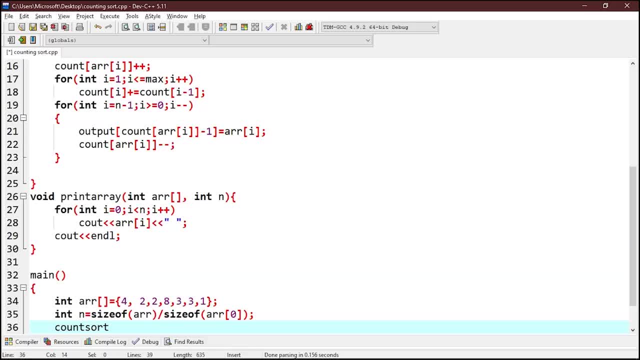 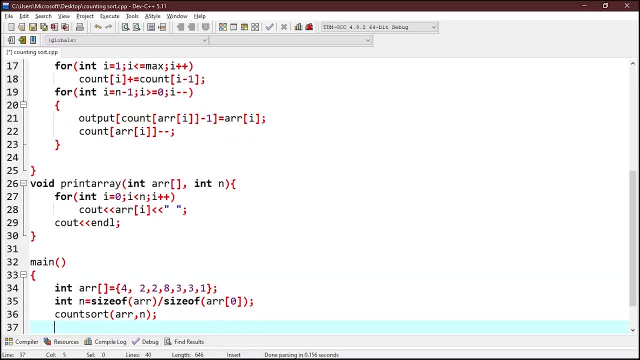 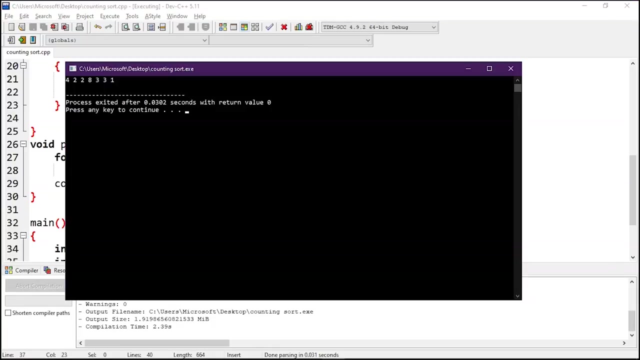 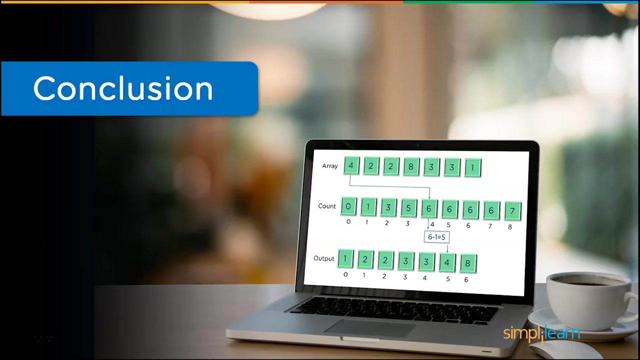 arr comma n. now we will print this array. so print array: arr comma n. now let's try and execute this. as you can see, we have successfully sorted this array using counting sort. let's try and execute this array using counting sort. let's get back to our slides. at last, let's sum up what we have learned. 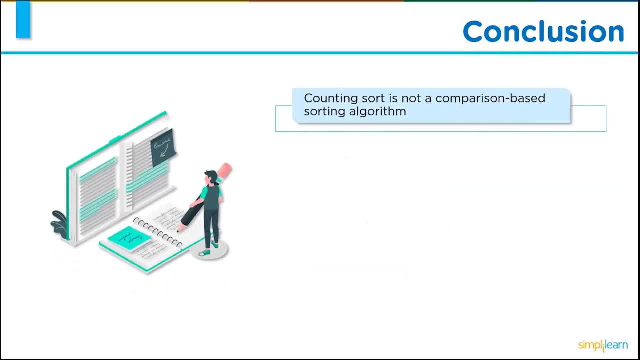 from this session. first up, counting sort is not an comparison based sorting algorithm. next up, it is frequently used as subroutine in other sorting algorithms, such as retic sort. next up counting sort can be performed only on positive integers. finally, counting sort utilizes a partial hashing to calculate the data item occurrence.